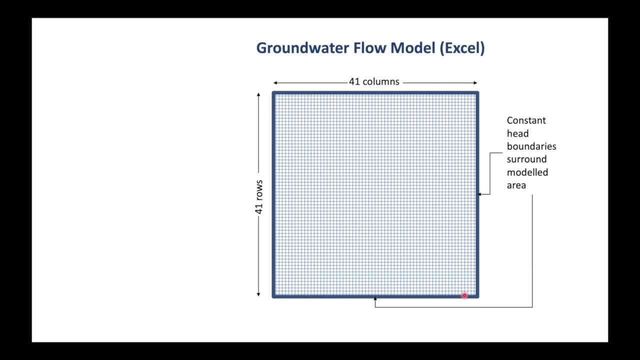 constant head boundary. This represents that large body of water that we talked about earlier. So basically, in these cells the hydraulic head of the water will always be constant. We can also change the cell size, and we do that in here. We just add the value. 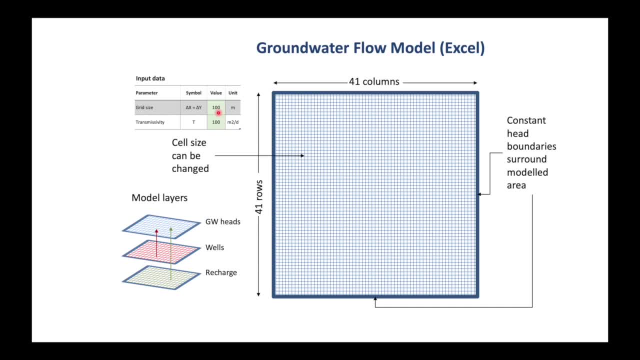 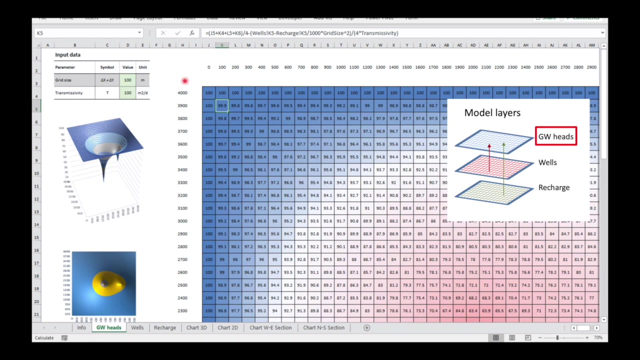 of the x and y distance and also the transmissivity. Our model has three main layers. One is groundwater heads, another one is called wells, where we can put in pumping wells, and the last one is recharge for groundwater. recharge In our groundwater heads layer is where we can change our grid size and also the 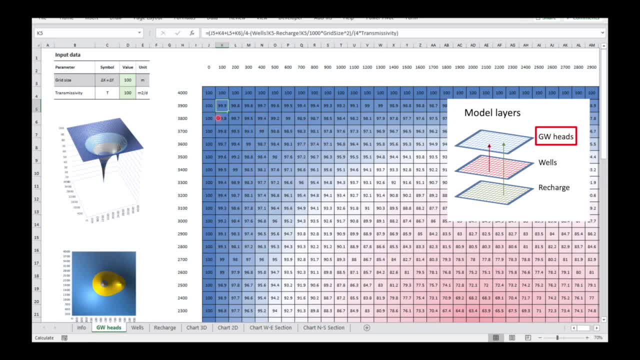 transmissivity, and you can see that the numbers which are calculated by the model will also be color-coded, so that the higher ones are in blue and the lower ones are in red. Let's go to the wells sheet. This is where we're going to enter. 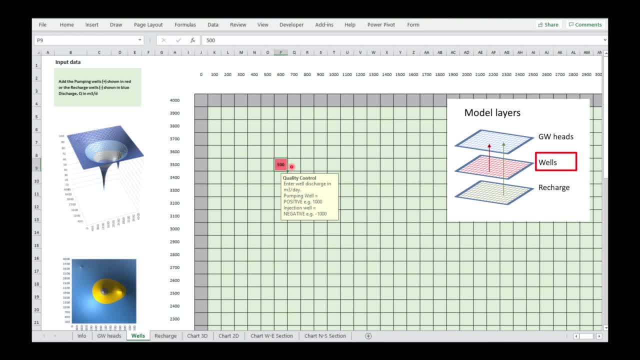 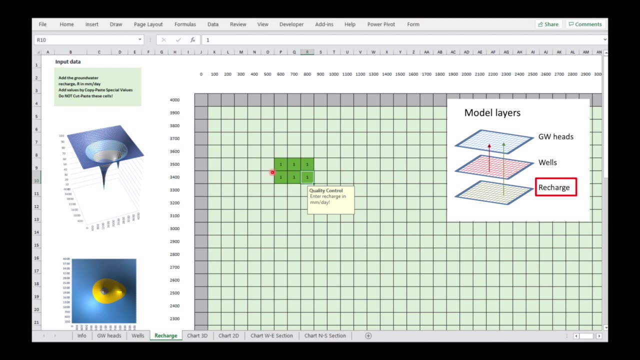 the wells and also the pumping rates in cubic meters per day. We can put in a positive number if it's a pumping well and a negative number if it is a recharge well. The last layer is the recharge layer, where we enter our groundwater recharge in millimeters per day, For example. here one means one. 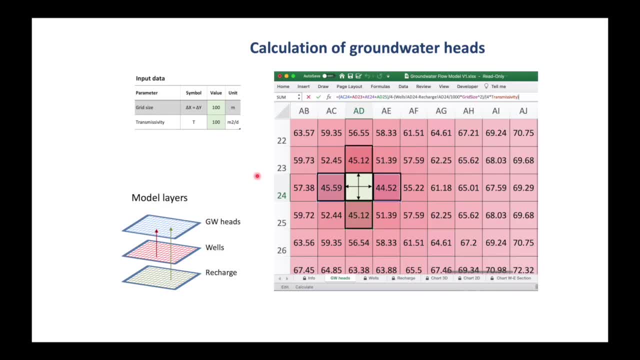 millimeter per day. What happens is that in the groundwater heads sheet the heads are calculated based on the heads of the surrounding cells and the also if there's any water leaving the cell through wells or coming in through recharge. Notice, here it's divided by a thousand because our recharge was in. 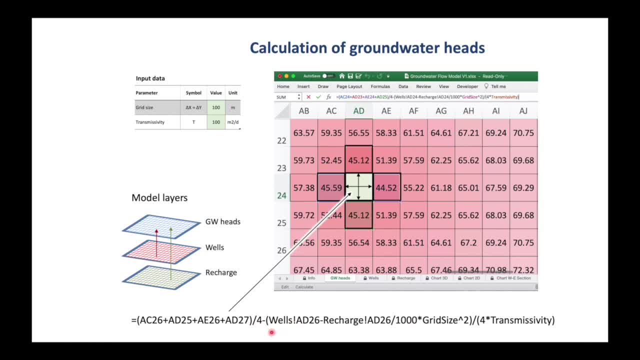 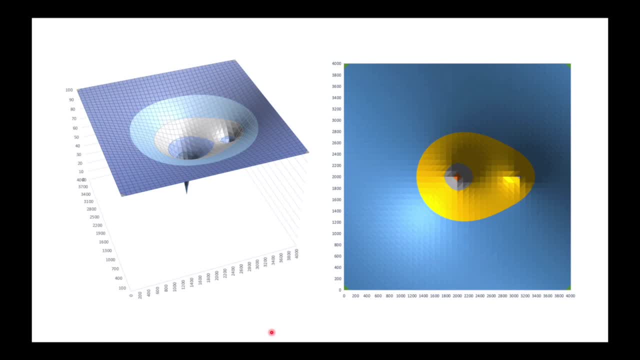 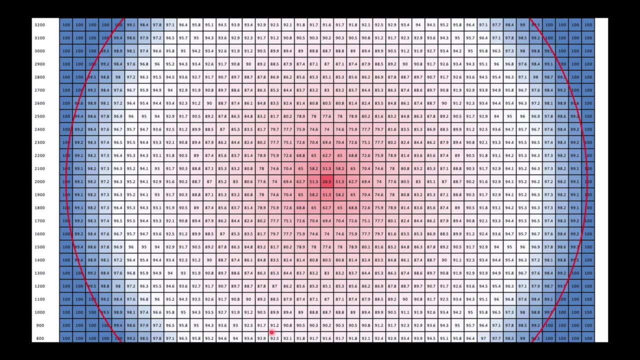 millimeters and we have to be consistent with the units here. Everything is in meters and days, And here are some of the results that we can produce in 3D and in 2D and also some sections to see what it looks like. Of course you'll ask: is this? 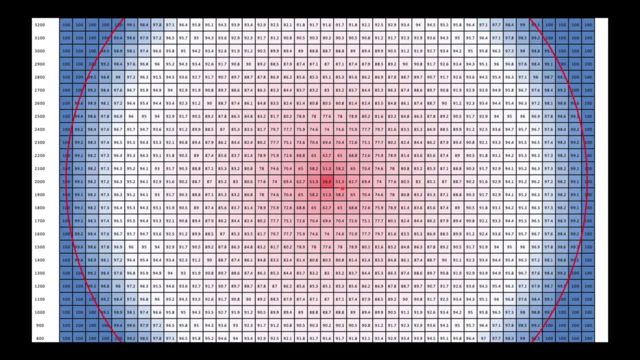 model any good? How does it look? How accurate is it? Here I've put a well right in the center of the model and at this fixed distance, here shown by the red line, I've entered a hundred meters into all the cells so that they're all constant head cells surrounding are well. 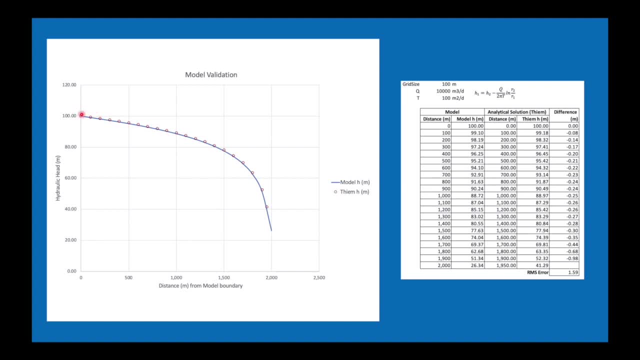 at the same distance And this is what the model has calculated. So at the outside we have a hundred meters of head and it decreases up to about 24 or so. and then we have a hundred meters of the center, where the well is, The red circles. 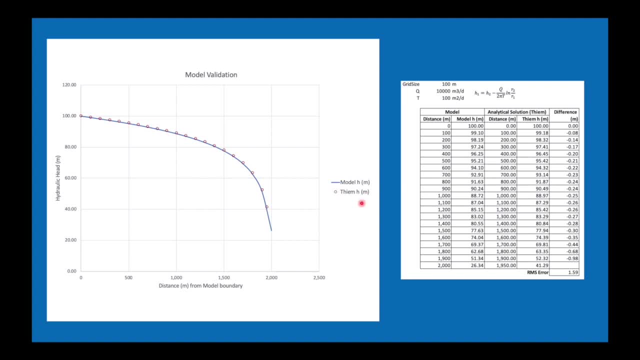 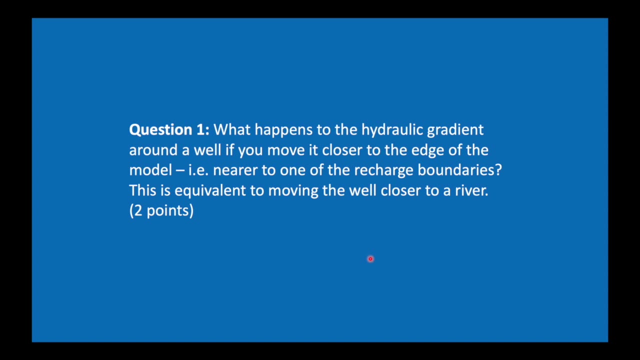 are what we calculate using the team equation, and actually the fit is pretty good. The reason it's a little bit different is because, of course, it's very difficult to make a round circle when you just have little square cells. Okay, let's move to our first question: What happens to the hydraulic gradient around? 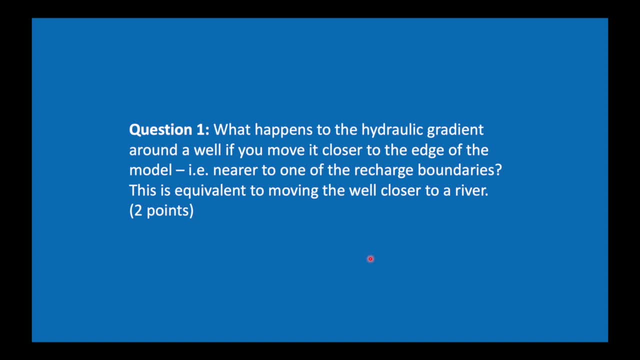 the well if we move it closer to the edge of the model, That means if we move it nearer to one of the recharge boundaries. This is equivalent to moving the well closer to a river. So here we are in our spreadsheet model. We're in the well. 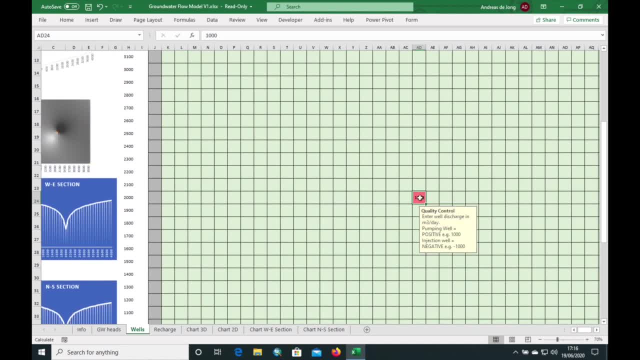 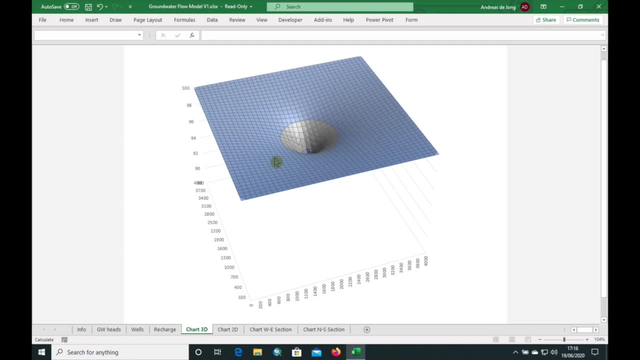 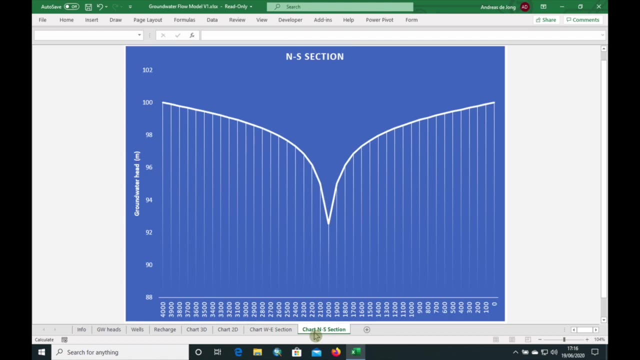 sheet and there is a well right in the center of the model pumping at a thousand cubic meters per day, And in 3D you can see the cone of depression around the well, also in our 2D section, in our east-west section and in the north-south. 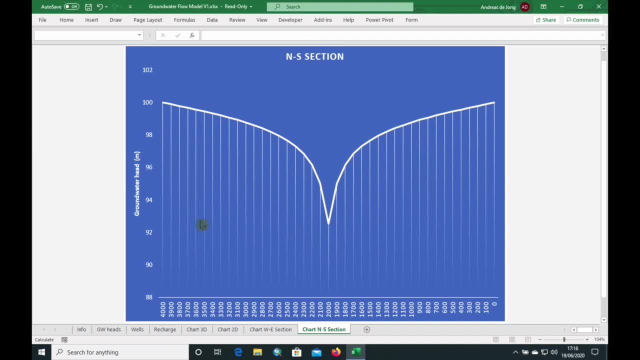 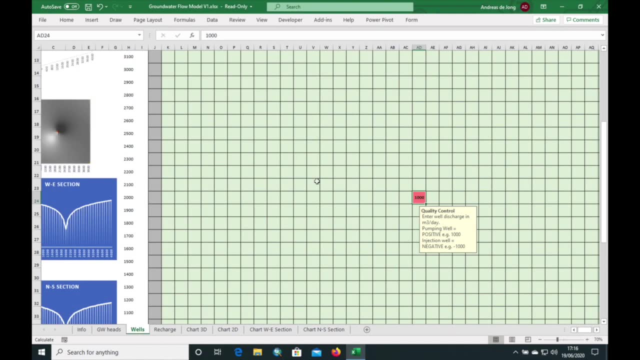 section. So what we're going to do now is we're going to move this well closer to the edge of the model where there is a constant head boundary. So I'm going to just randomly put in a thousand kilometers per day here and take away 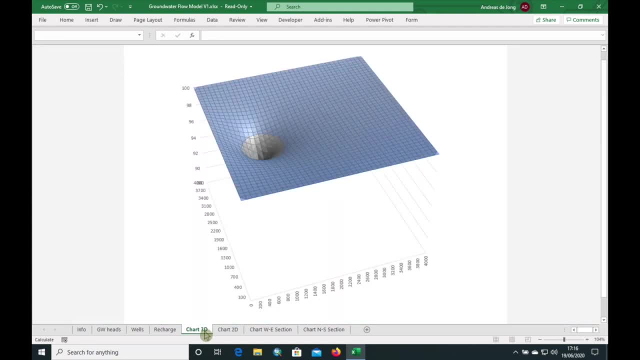 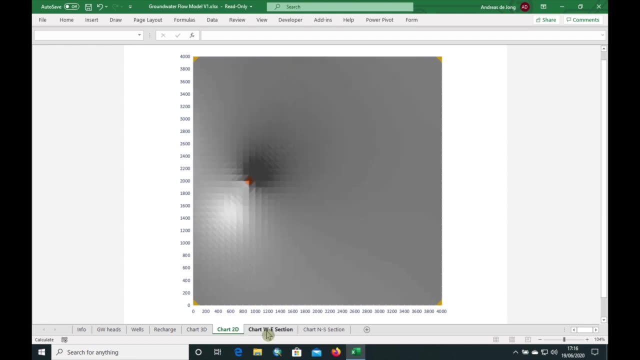 this one And let's have a look. Oops, It is moved close to the edge and you can see how the gradient has increased here And also in our sections. Okay, that one doesn't move too much, because we're actually moving along a. 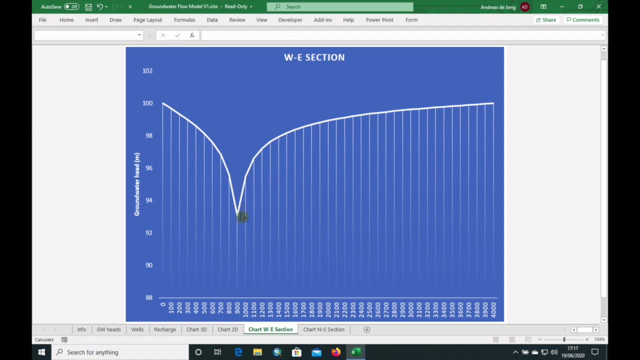 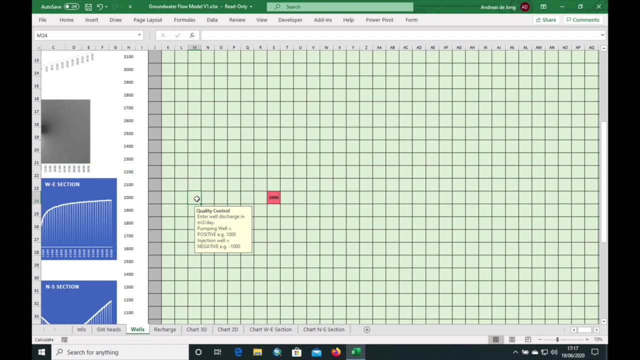 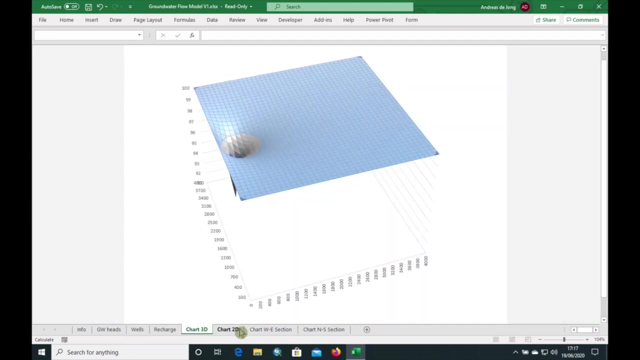 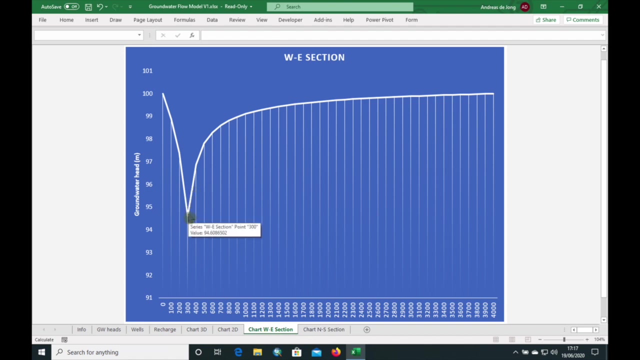 west-east line. So you can see as we move the well closer to our recharge boundary, the gradient gets steeper, closer to the recharge boundary and the gradient becomes less steep on the other side. Let's move it even closer And you can see as we get closer and closer to the recharge boundary. the 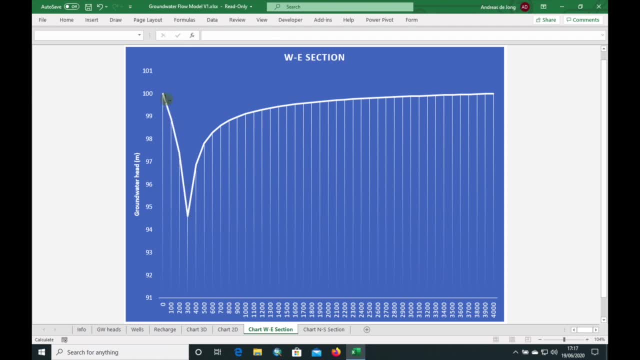 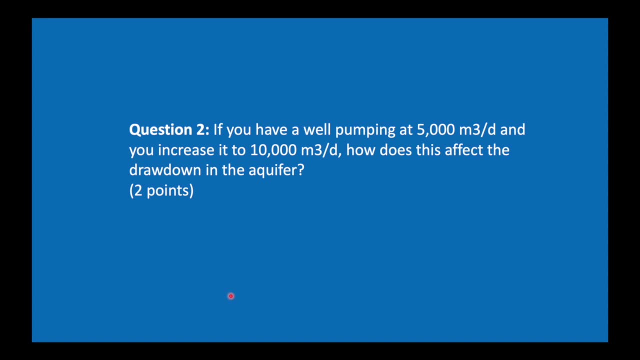 gradient has to become steeper, because of course here the constant head boundary cannot change. If we have a well pumping at five thousand cubic meters per day and you increase it to ten thousand cubic meters per day, how does this affect the drawdown in the aquifer? Okay, first of all I need to 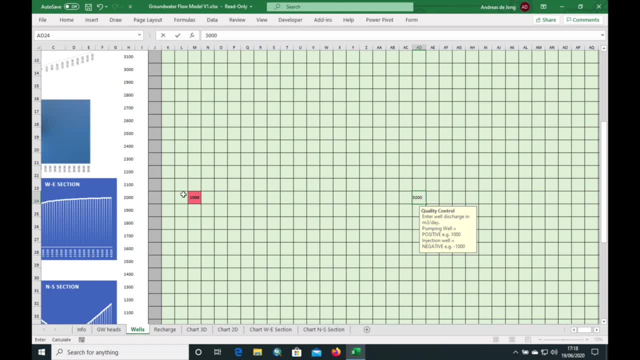 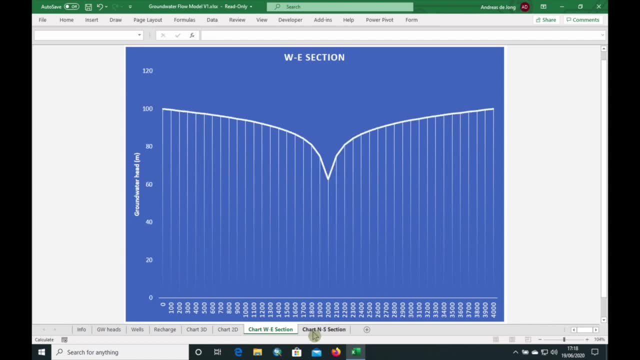 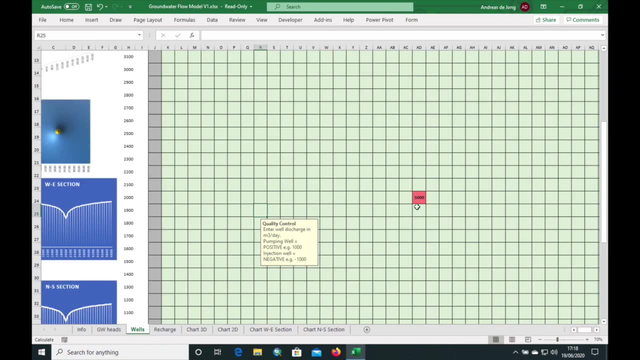 move this one well close to the center of the model. so we have a well pumping at five thousand cubic meters per day in the center of our model. There we go, and now I'm going to have a look at our groundwater heads. first of all, We have a 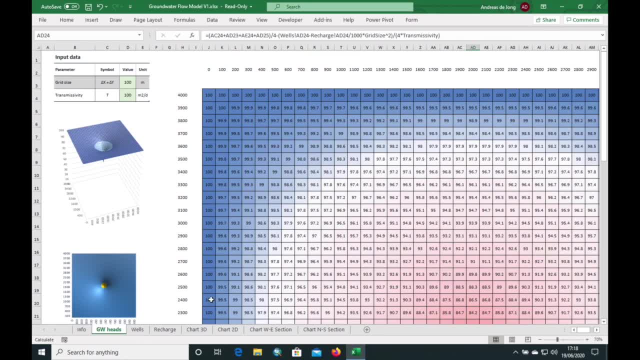 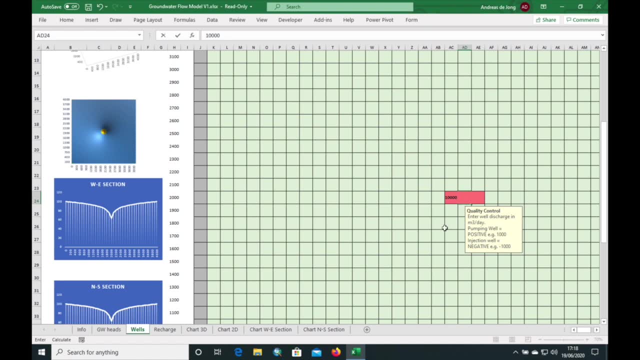 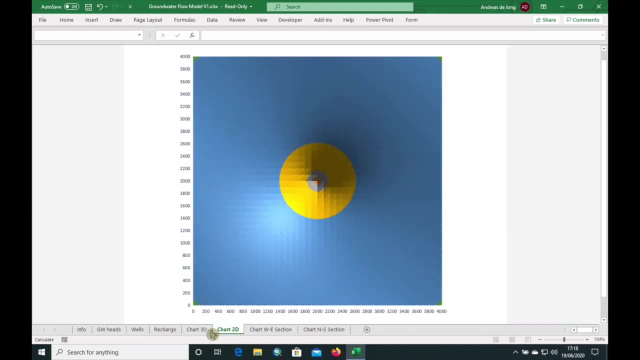 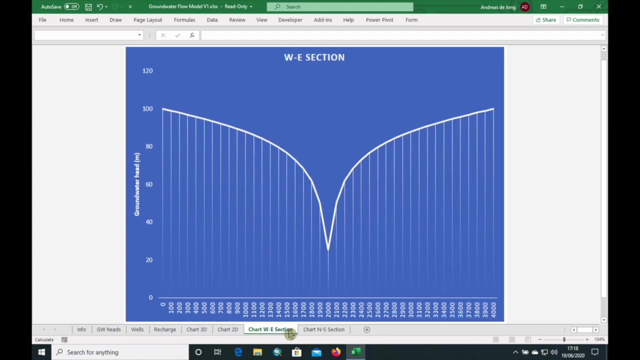 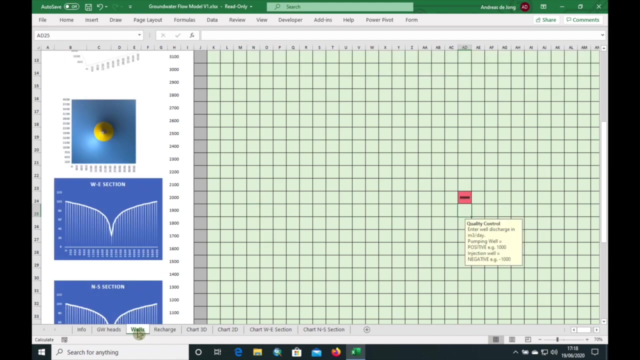 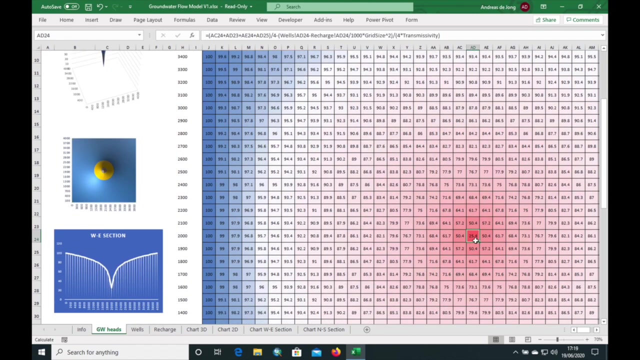 head of about 63 meters here Now the. So the question is: what happens if we increase it to 10,000?? As expected, the drawdown increases quite dramatically, And it's now at only 25 meters. If I was to increase this even further, maybe we'd even dry up our model. 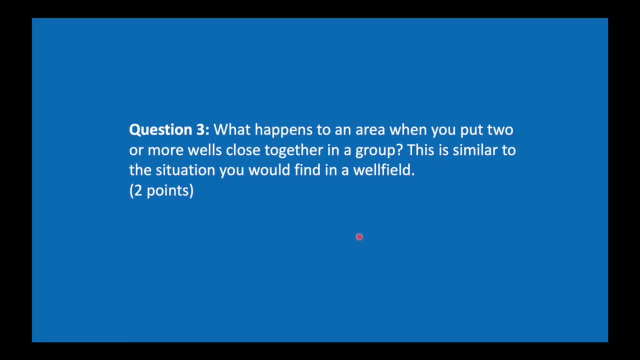 So we won't do that at the moment. Okay, let's move on to question number three. What happens to an area when you put two or more wells close together in a group? This is similar to the situation you would find in a well field. 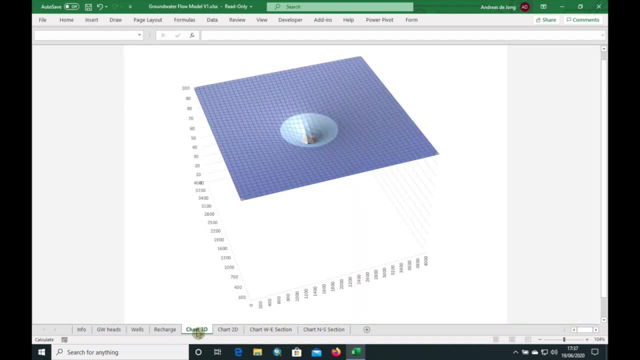 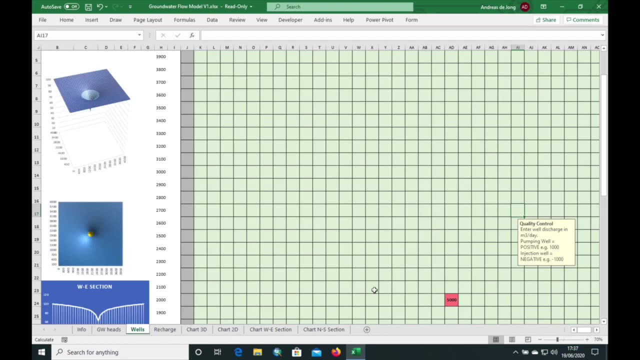 So at the moment, we have a single well in the center of our model, With a simple cone of depression around it, And we're going to add some additional wells, So let's add another one here, And another one here, And another one here. 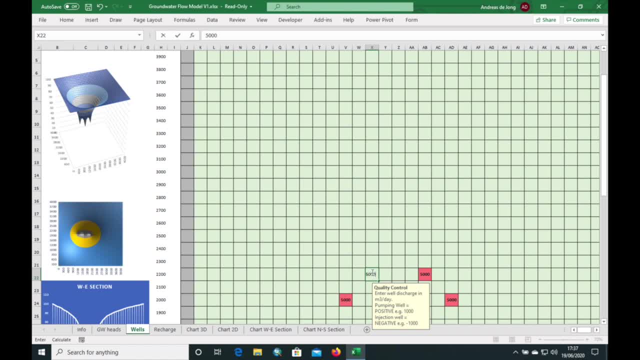 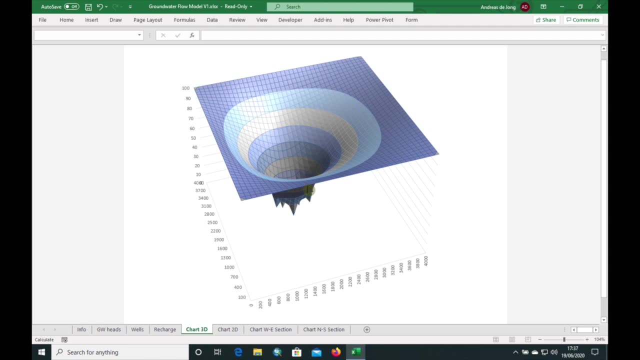 Another one here. You notice that as we enter the numbers it is changing to red, So we can see that we added two wells. These are pumping water from that area And you can see that if we have more than one wells together in a group. 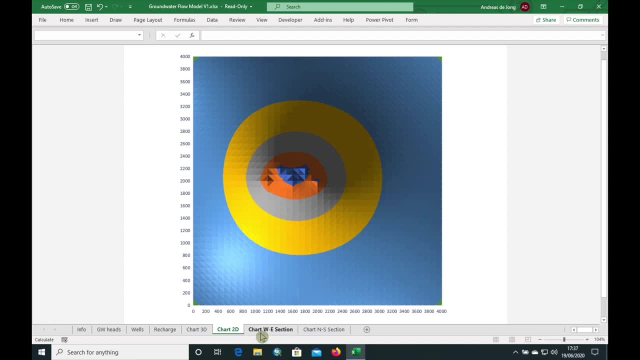 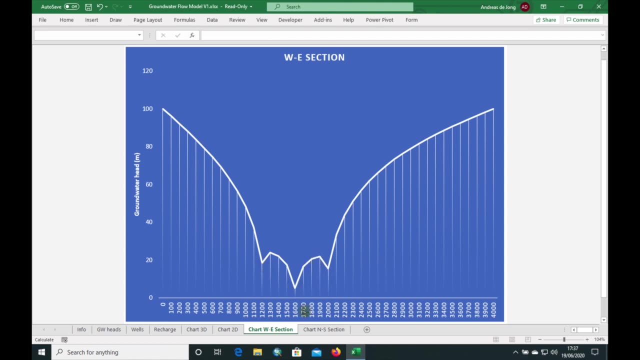 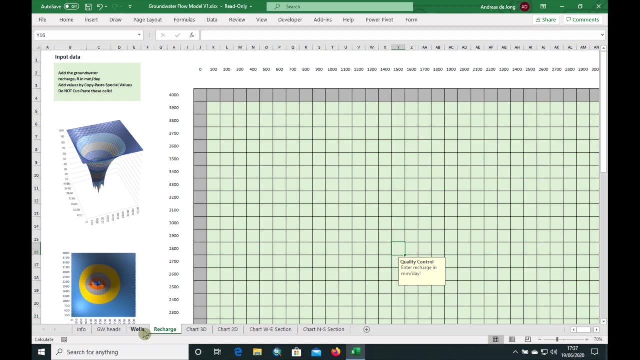 they basically create a much bigger cone of depression, Which can be simplified. Think of it as if there was one huge pumping well right here in the center of the well field. We have to be careful here, because we've almost de-watered the aquifer. 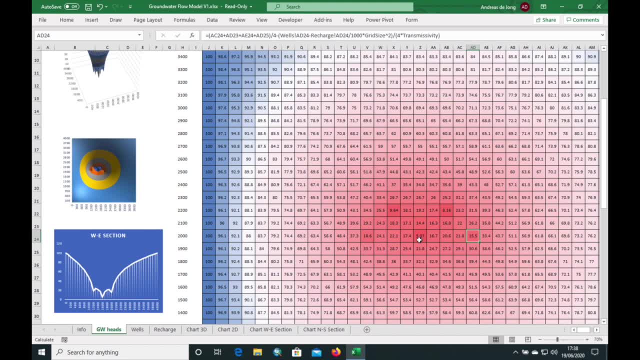 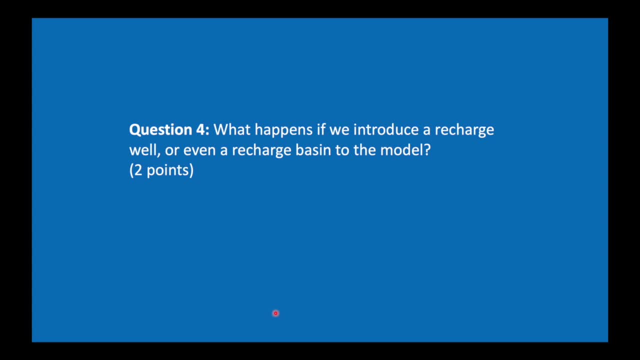 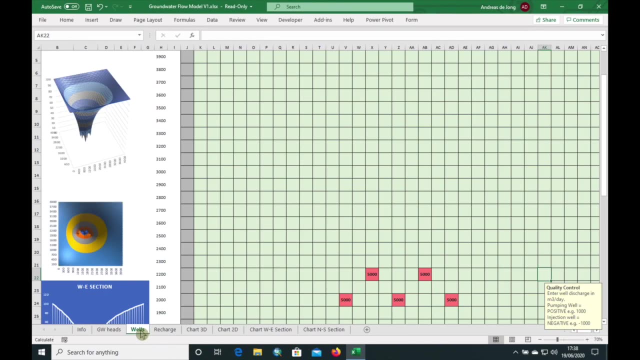 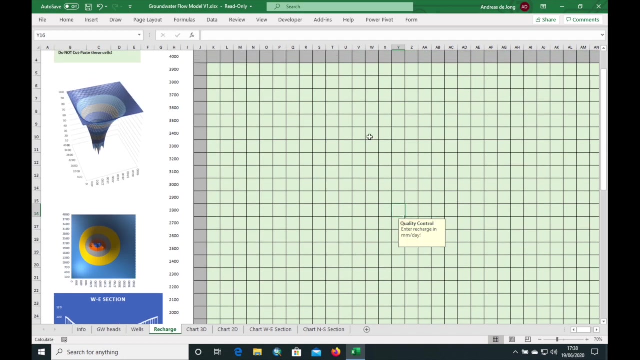 You can see it's only five meters, So that's getting really close. Next question: What happens if we introduce a recharge? well, or even a recharge basin to the model? So first of all, let's see what happens if we add a recharge basin up here somewhere. 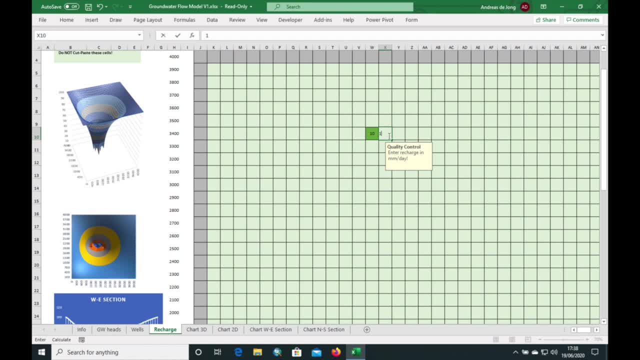 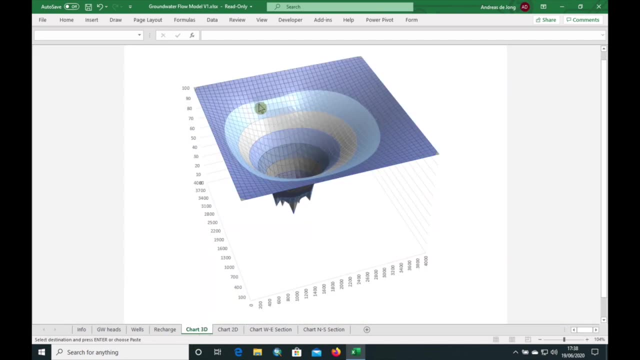 We're going to say we're going to recharge at 10 millimeters per day And actually what I can do is I can copy and paste. Let's have a look. Ah, we can see the effect of the recharge basin. Not very much. 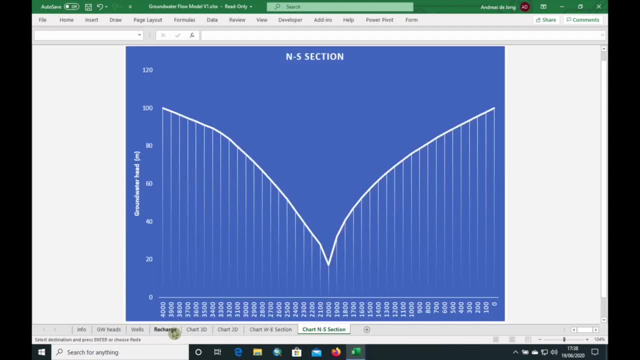 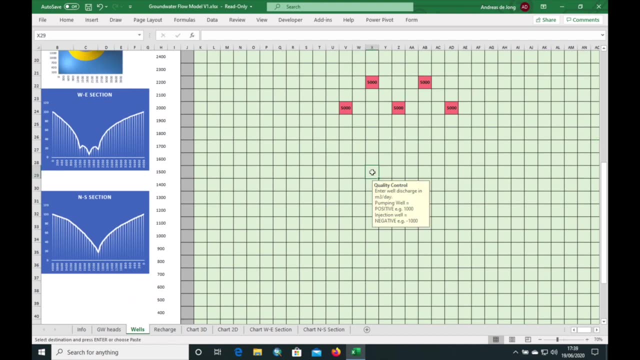 But it does lift the groundwater levels a little bit. Let's add some recharge wells Maybe here, And remember it has to be pretty low. So we put in cubic meters per day but negative because it's a recharge well And it changes colors. 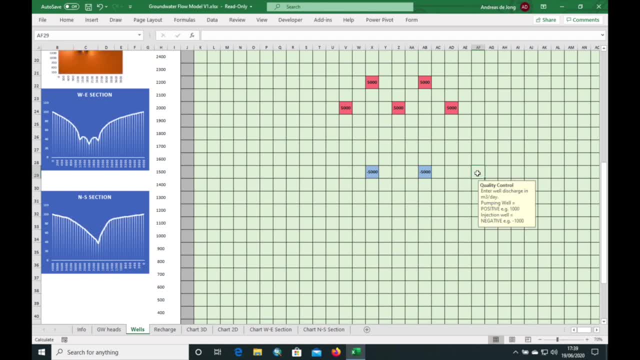 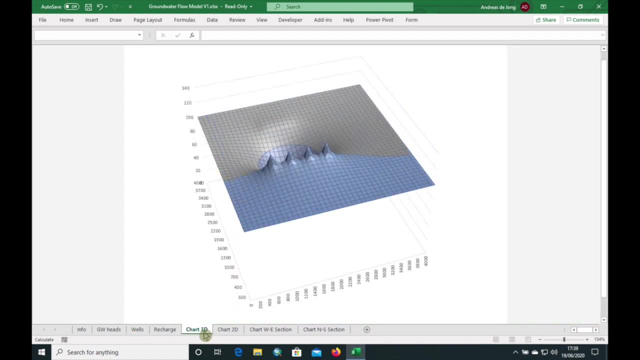 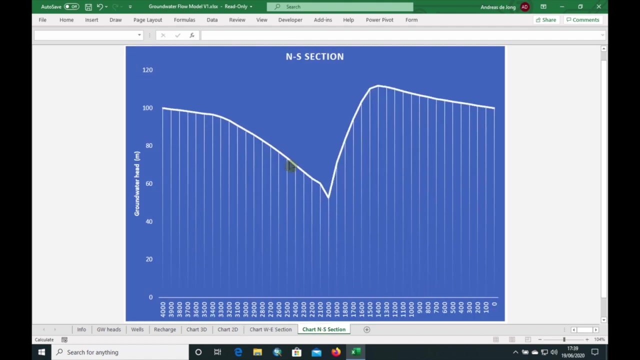 It becomes blue. to help us avoid making mistakes, I'm going to put a line of recharge wells here, Maybe another one here, Okay, And you can see the immediate effect here that the groundwater levels start to rise And here you can see, this is our effect of our well field. 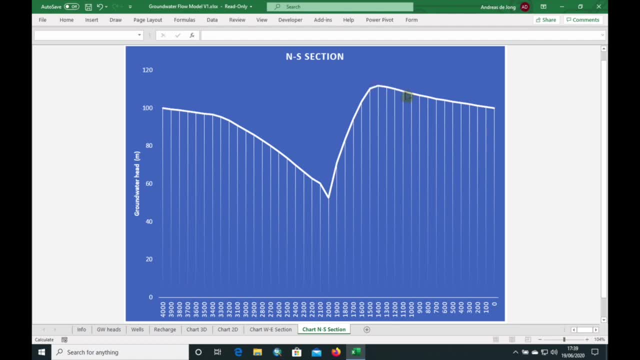 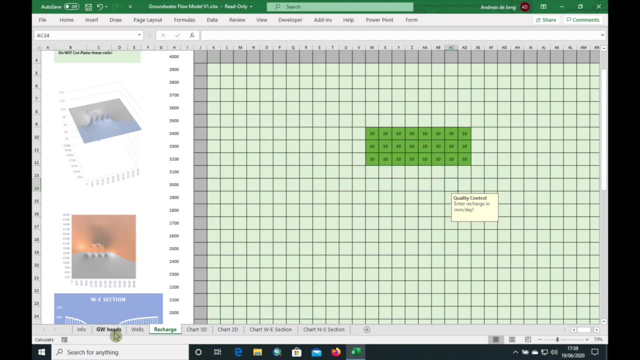 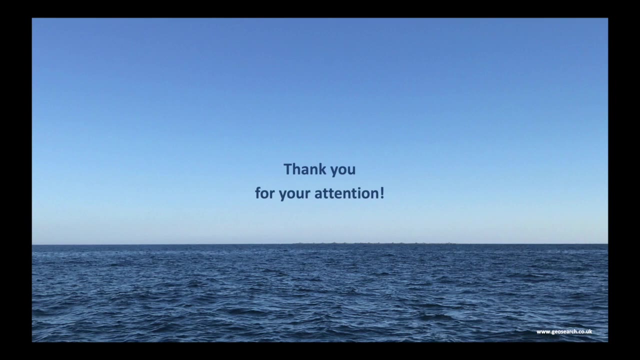 And this is the effect of the recharge wells, which basically do the opposite to that cone of depression. That's the end of our questions, So I hope you enjoyed it And thank you very much for your attention. Keep playing with the model And I think it's quite useful to understand groundwater flow in an aquifer.